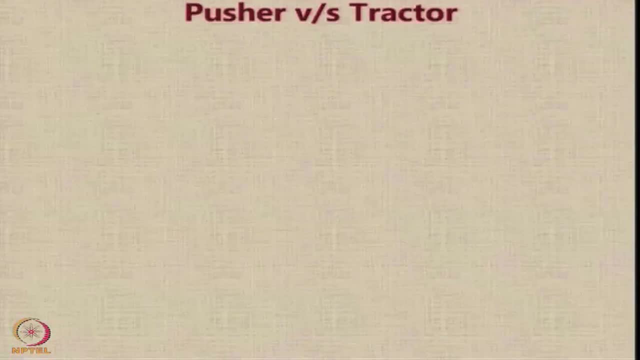 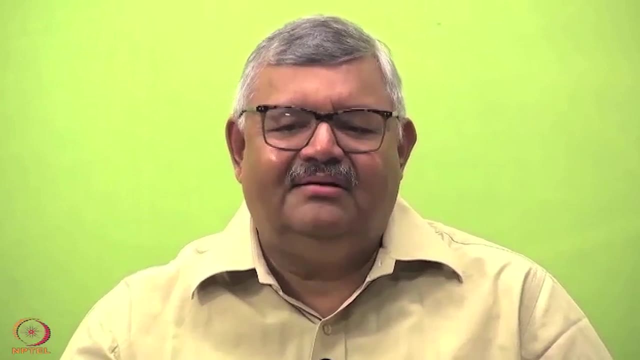 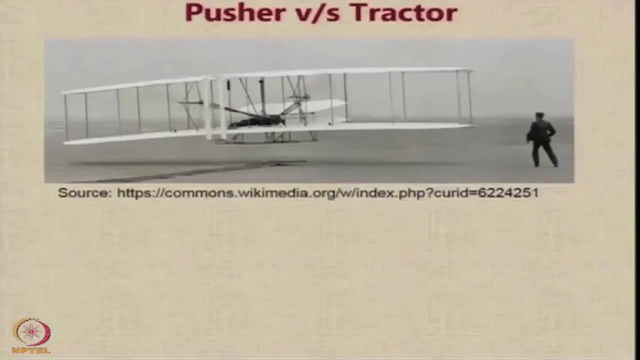 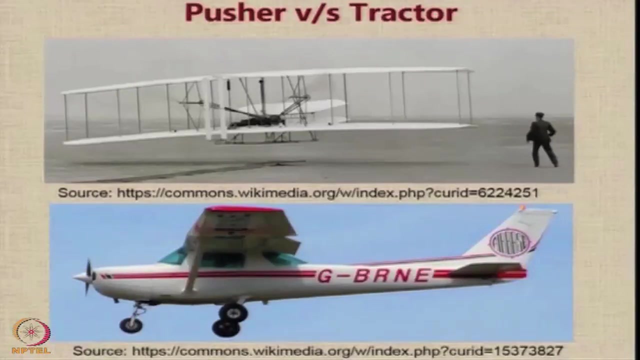 tractor configuration. The pusher configuration is very is considered today as uncommon and special But interestingly, the first aircraft to fly successfully, the Wright Flyer of 1903, was a pusher configuration And most of the aircraft which are used today that are meant. 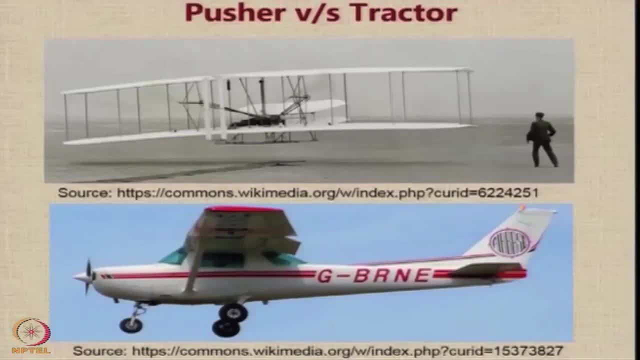 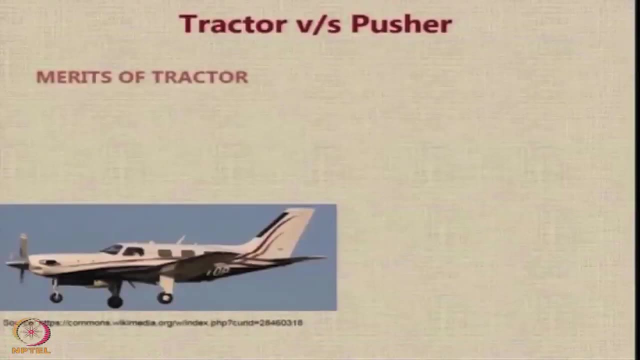 for training of pilots or general aviation. Typically, such aircraft have a nose mounted engine and they belong to the family of tractor propulsion. Each category has its own advantages and disadvantages. Let us have a look. Let us first look at the merits of the. 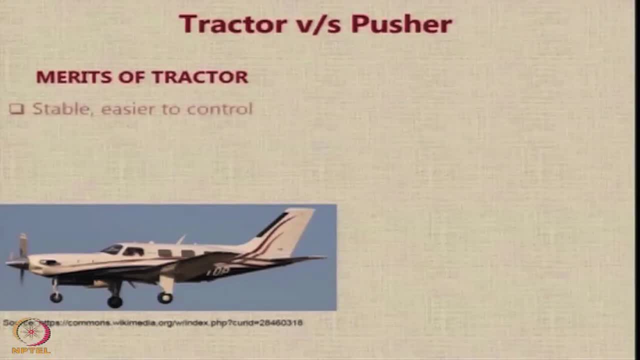 conventional configuration or the tractor configuration. The first and the most important factor is that a tractor configuration of engine gives you a configuration that is stable and relatively easier to control Because the propeller is in undisturbed flow, facing the wind as the aircraft flies forward. you get higher propeller efficiency And, in most cases, 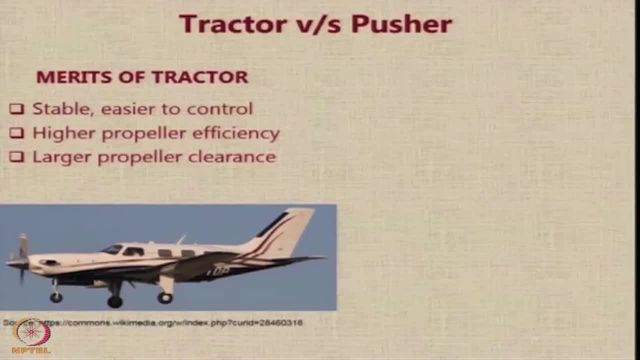 you can also get much larger propeller clearance. This is especially true for tail wheel type of configurations, where the propeller in the nose gives you more clearance with the ground, And the air which the propeller throws on the fuselage can be used to cool the engine. So most tractor engine configurations have air cooling of the engine. 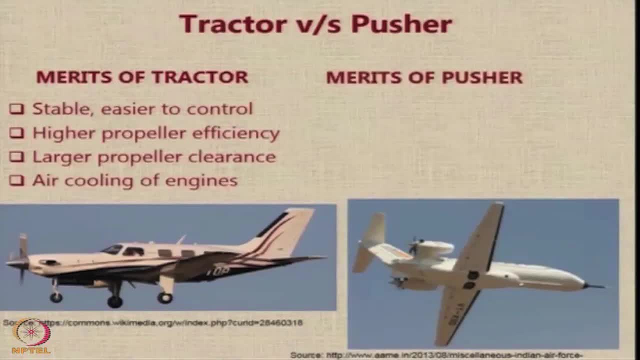 engines. On the other hand, we have a pusher configuration like the one shown here. This is the Saras aircraft, designed by National Aerospace Laboratories, Bangalore, which has two engines mounted on the back and behind them we have these propellers. So this is a pusher configuration because the engines are behind. 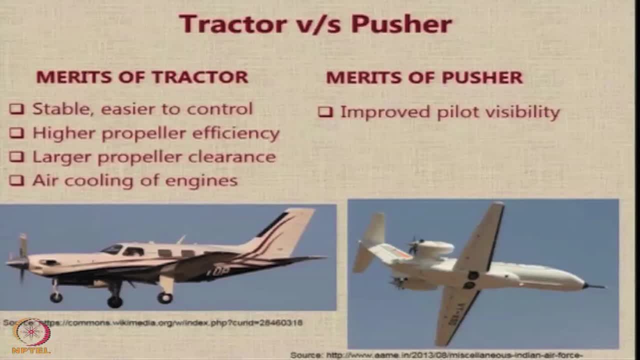 You notice here that since the engines are quite far away from the canopy, therefore you have unrestricted improved visibility for the pilot. the prop does not come in the way. And the second thing is pilot safety, In case there is any problem with the engine. 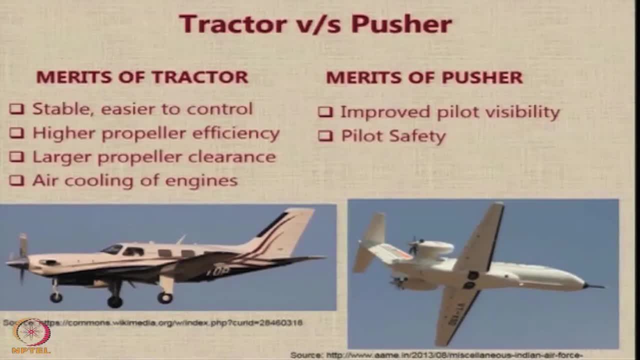 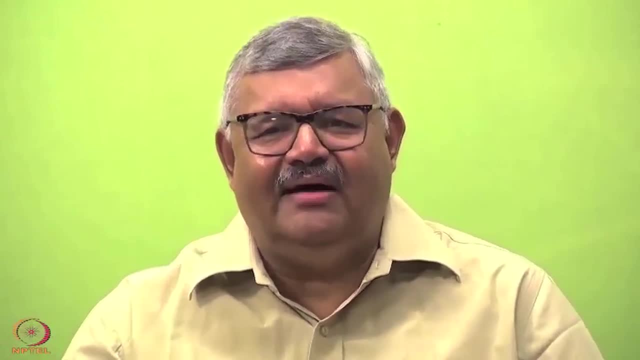 this was very common in the earlier days when engines used to catch fire, And if you have engine right in front of the pilot and if there is a damage or if it catches fire, then the whole problem will be immediately passed on to the passenger case. 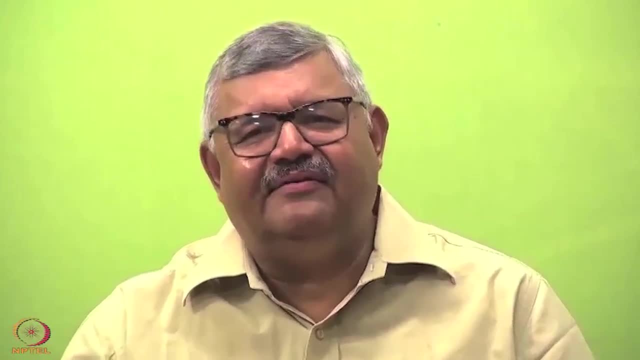 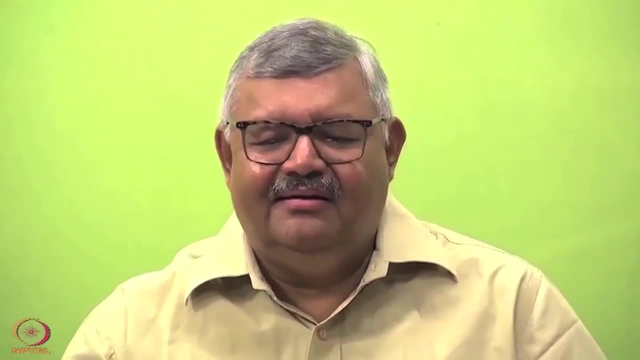 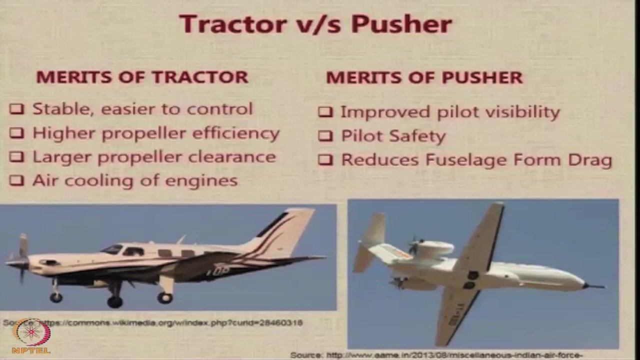 So, from pilot safety point of view, it is better if the engines are far away and behind you, so that, in case of any problem with the engine, the pilot is not directly injured or affected. Another important point is that the pusher configuration, which normally has the ability to wash away the disturbed air which is flowing over 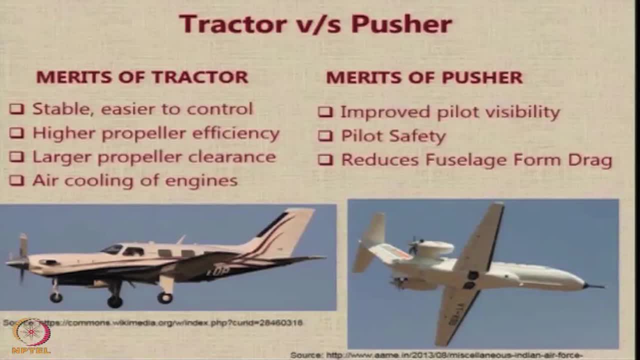 the rear fuselage, behind the wing, due to the wake of the wing. it can energize that air and with that it can reduce the form drag of the fuselage. And lastly, a pusher configuration in which the propeller is mounted behind the wing of the aircraft. you leave the wing in completely. 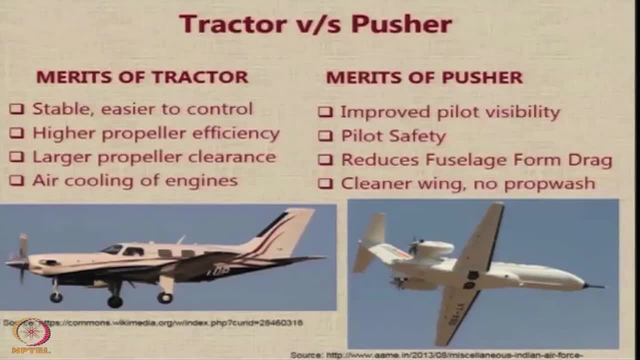 undisturbed flow of the air. In the tractor configuration, the propeller is throwing swirling air on the fuselage and it can create a large amount of drag. It can lead to separated flow, Whereas in the case of pusher, the engine is mounted behind. Therefore, 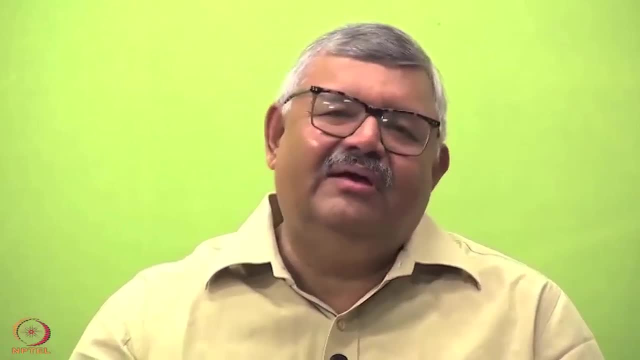 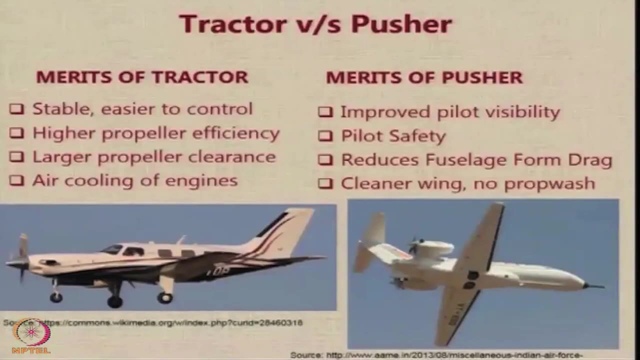 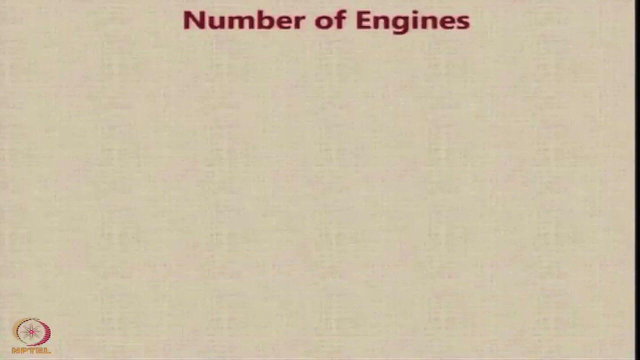 it is actually sucking air over the wing And hence the wing gets very clean, undisturbed air with no propeller wash. So depending on which configuration is of use to you, you have to choose an appropriate one. As far as number of engines is concerned, there is no clear-cut indication from any accident. 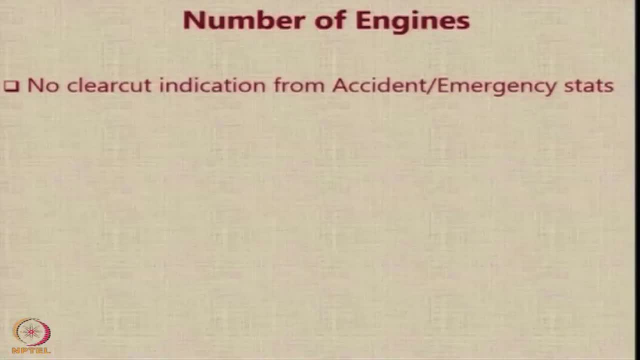 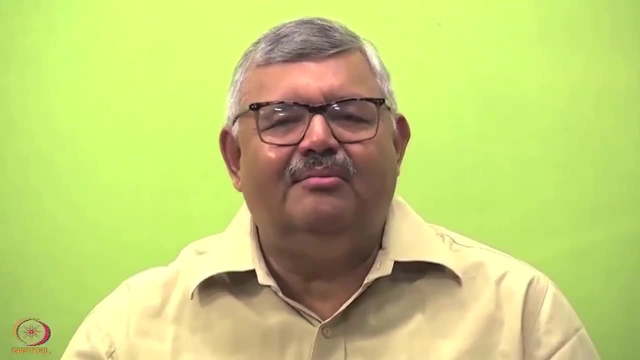 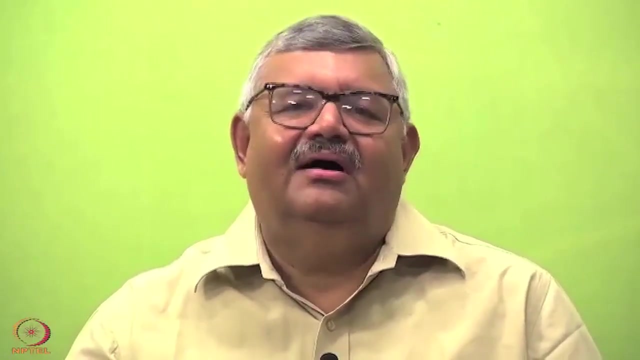 or emergency statistics. There have been equal number of accidents when the aircraft is with two engines, or with three engines, or with four engines. So having more engines, more than one- see more than one- is essential because you need to have redundancy and therefore you need to have at least two engines, especially when you carry a fair amount of passengers. The regulations are very clear on this. The moment you carry nine or more passengers who are fare paying passengers, you are required by law to have more than one engine and most.